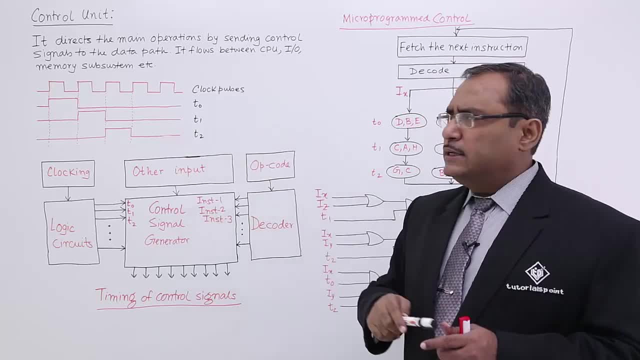 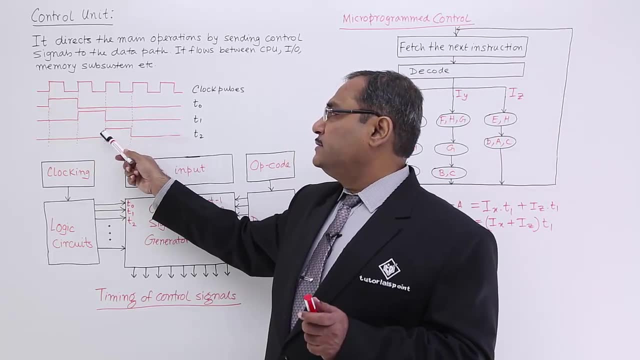 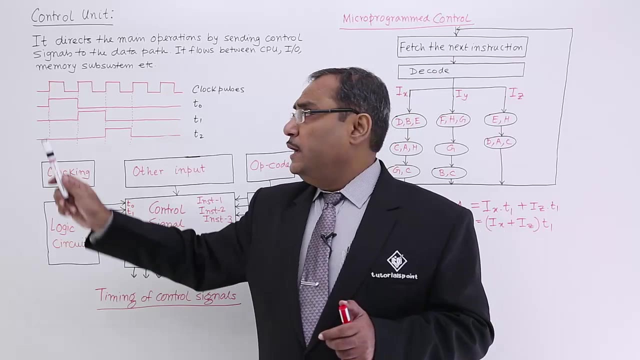 issues. ok, So now for a example, you can say that this is the clock pulse and you see, this is the first cycle, this is the second cycle, this is the third time period, and so on. So first, second, third, I am marking them as T 0,, T 1, T 2.. In the first case it 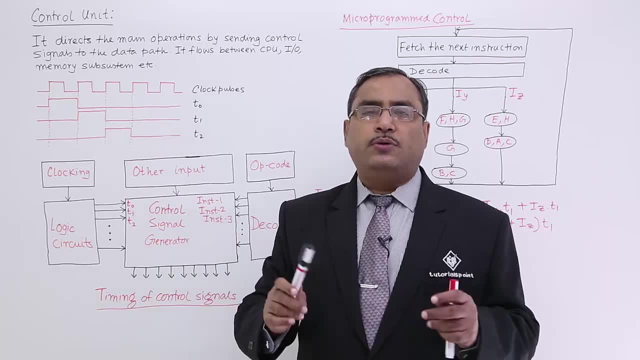 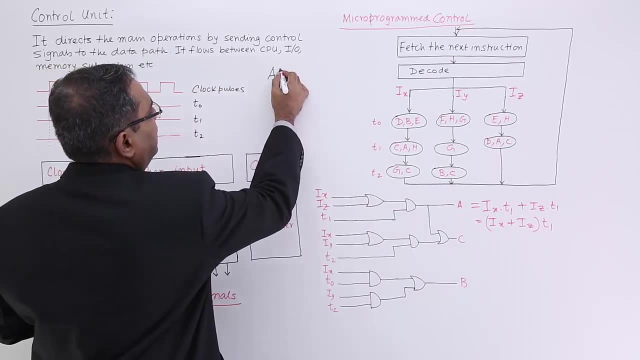 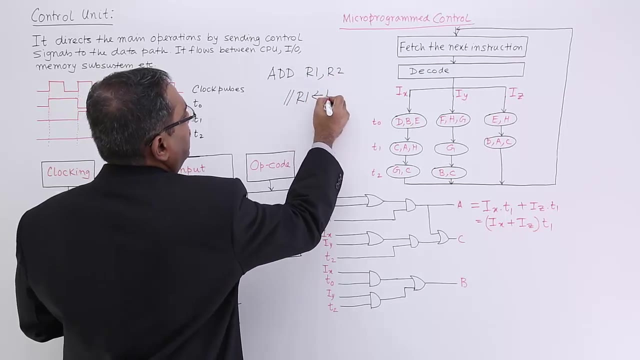 will do something. in the second cycle it will do something and so on. Say for a very simple example, I can tell in this way: let us suppose that is one instruction called say What does it mean? Means R 1 will get initialized by the current content of R 1 plus the current. 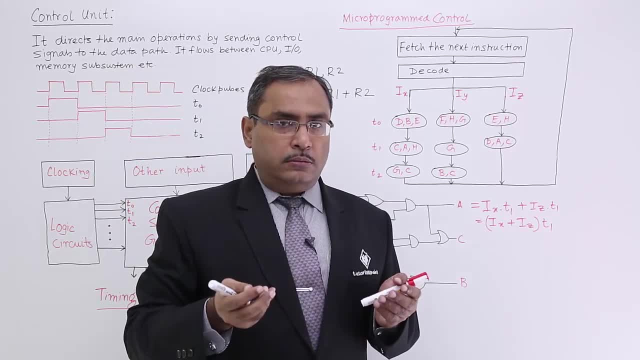 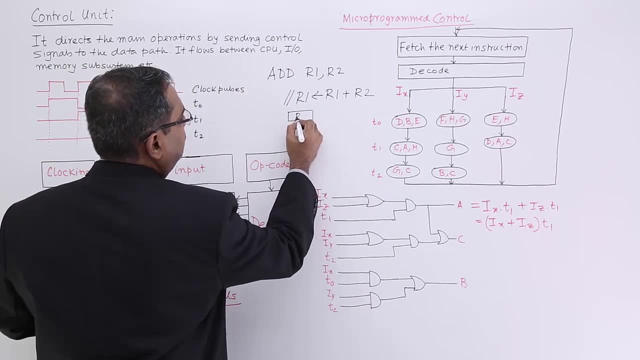 content of the register R 2.. Now how this circuits will be operating, Say I can show in this way: let us suppose there is a register R 1, there is a register R 2. So at first I should select this register in the read mode. 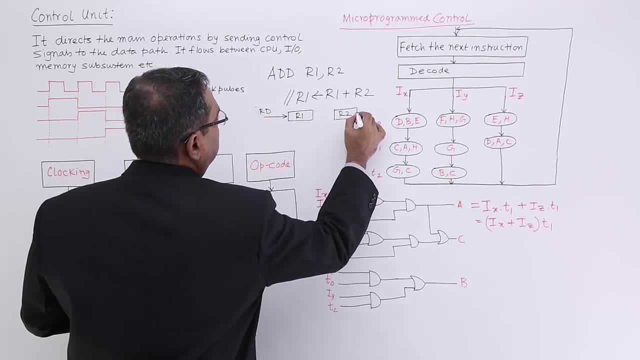 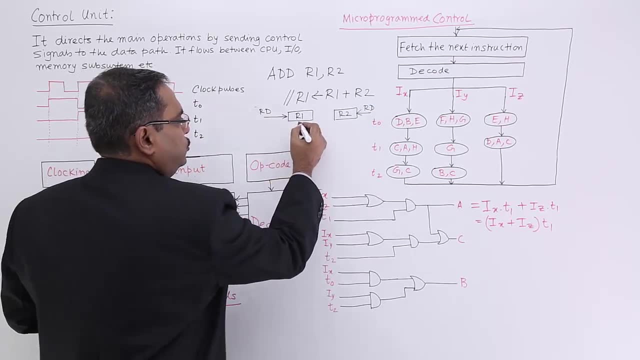 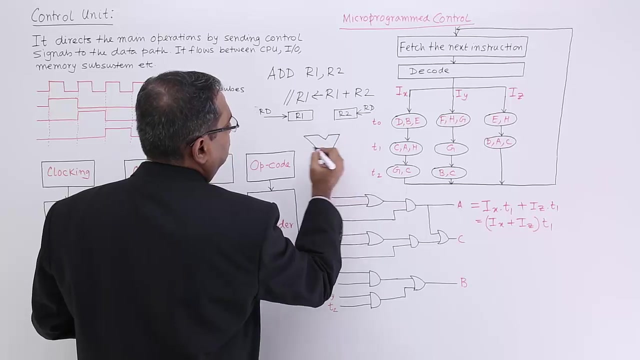 I should select this register in the read mode and also this register in the read mode. I am just giving you a very simple example. So from this register's content, let us suppose this is my ALU, This is my ALU, where the addition operation will take place, So data will be. 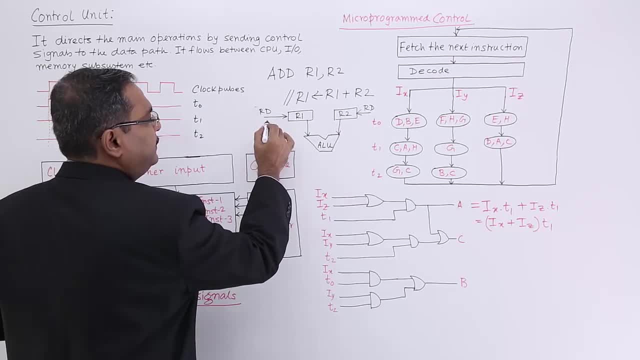 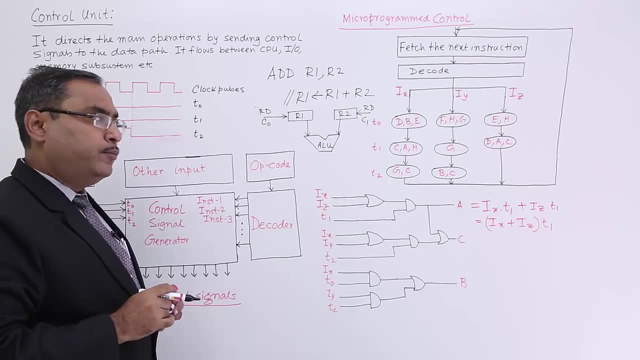 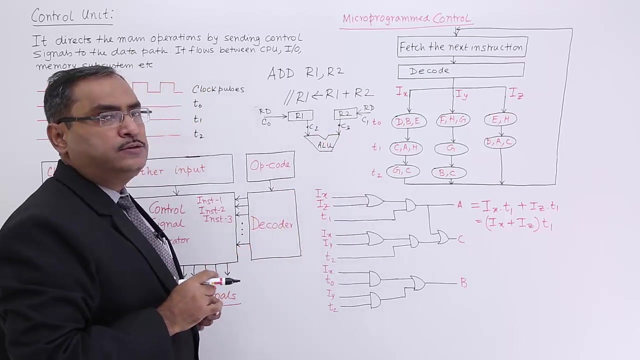 coming from register 1 and register 2.. So first time this control signal say C 0 and C 1 will be enabled to make the registers to be selected in the read mode. next time it will make this cell C 2 and C 3. these 2 control signals will be enabled to make the 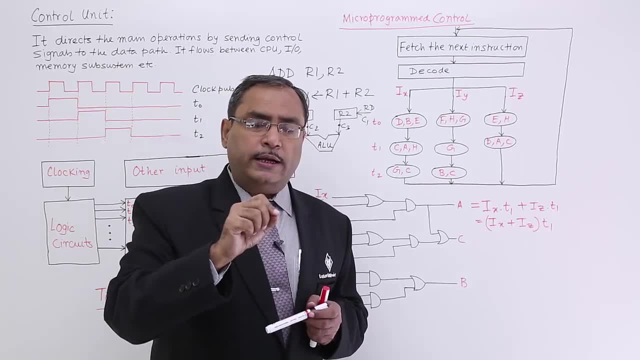 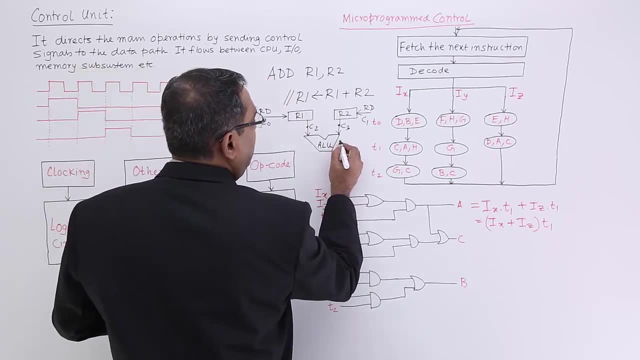 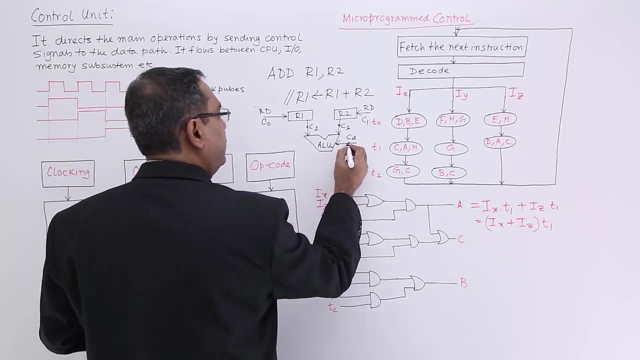 data path enabled so that the register 1 content and the register 2 content must be available to the inputs of the ALU, then the ALU should get enabled, say by the control signal C4: ALU. ALU should get enabled. So ALU will do the sum of R1's content and R2 contents because 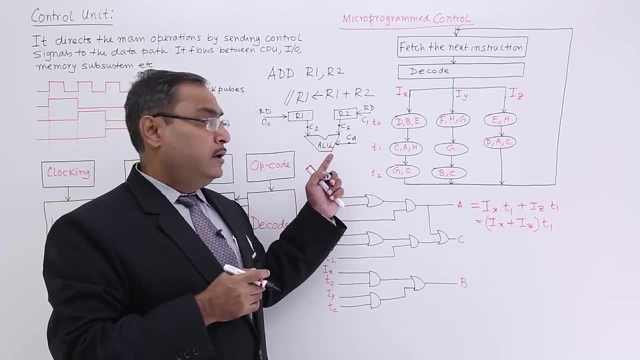 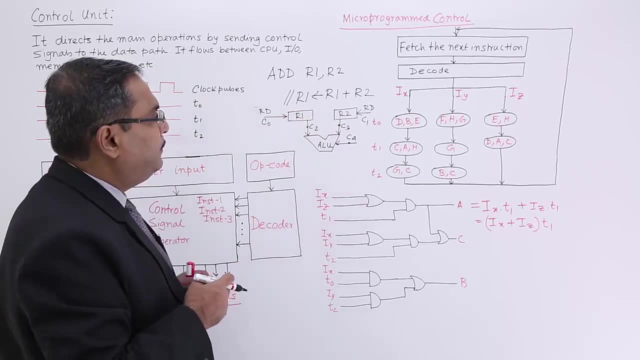 their contents are available through the data paths. Now, what will be the output? Output will be obtained from the ALU as a sum, So please tell me, where should I keep this output? I should keep this output to R1.. I should keep this output to R1.. So this output will be going to R1.. 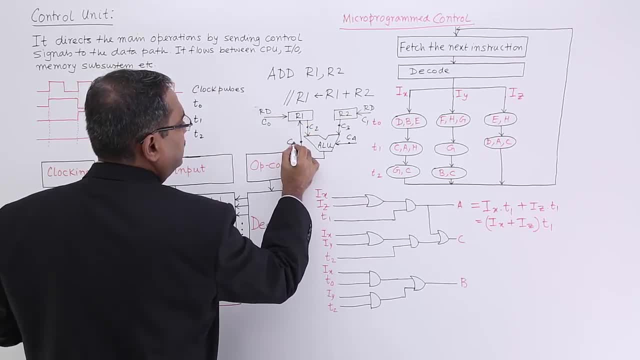 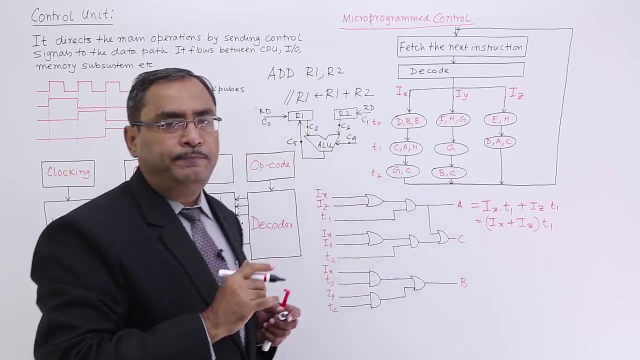 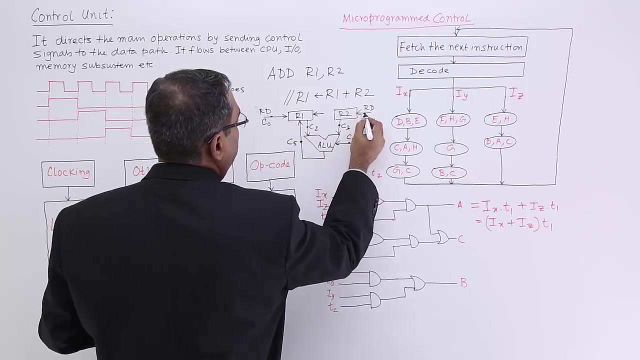 So again, another control signal, say C5, will be enabled, so that the ALU's output will be going to R1. And in the meantime also the another control signal will come into the play. So let it be C0,, let it be C1, C2, C3,, C4, C5. So let it be C6, which will make this register to be enabled. 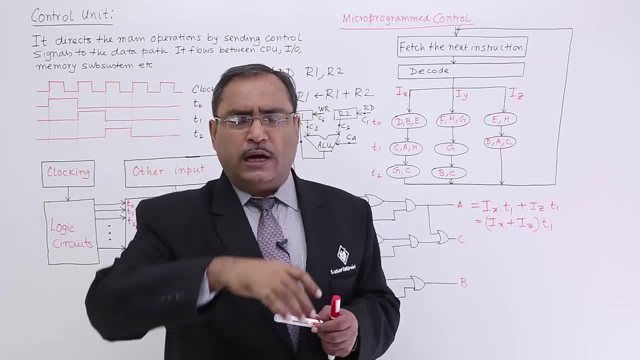 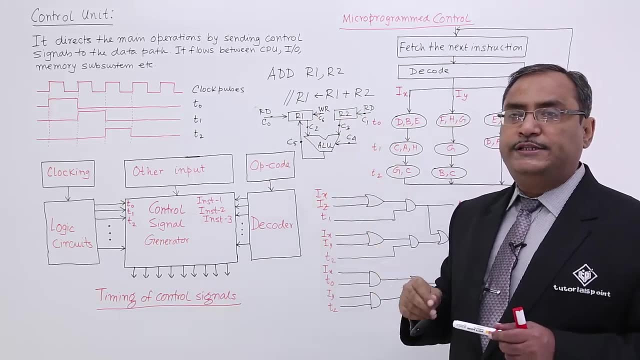 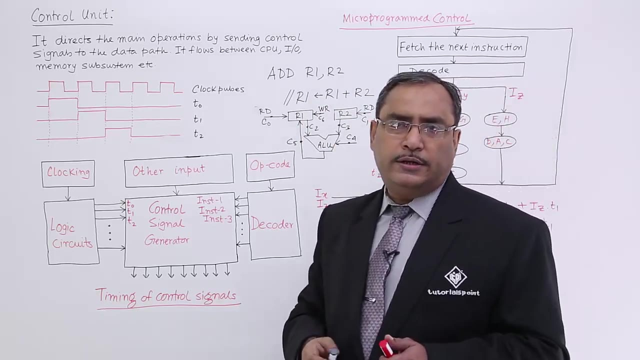 in the right mode And in the meantime, obviously, the other control signals have got disabled. So you see the sequence of control signals, how they should get generated so that this addition operation can take place. everything will be decided by the control circuit. Just think for. 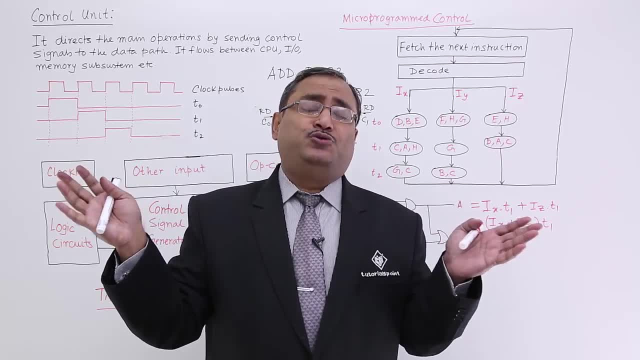 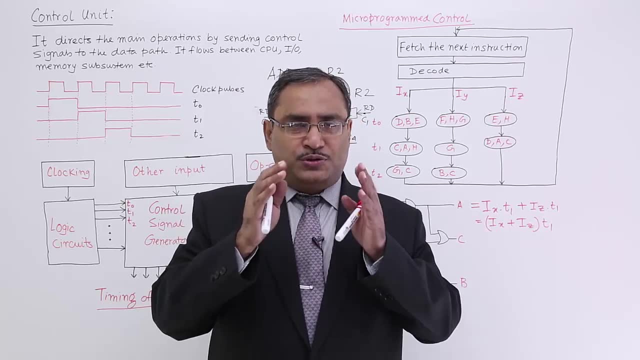 each and every processor, so many instructions are there, So many control signals are to be initiated, are to be enabled, are to be disabled. after this, before that. So think about the complexity of the control unit. But here, in case of computer organization, where there is 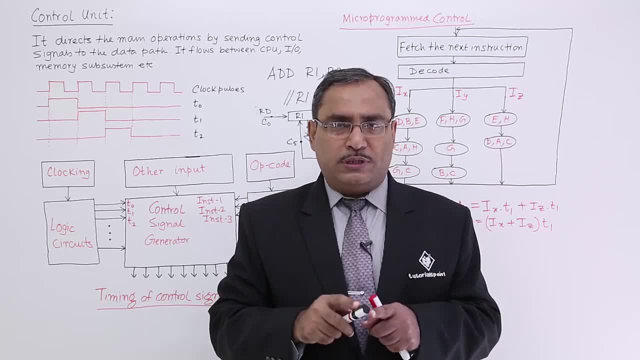 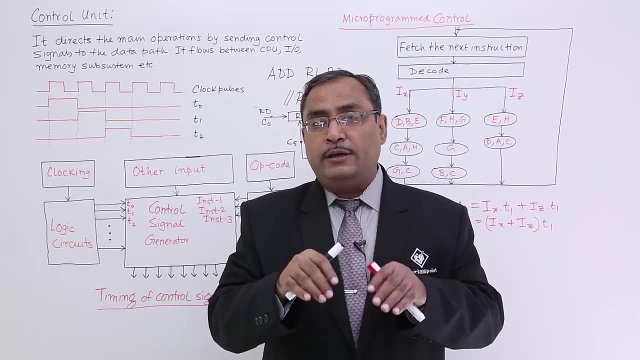 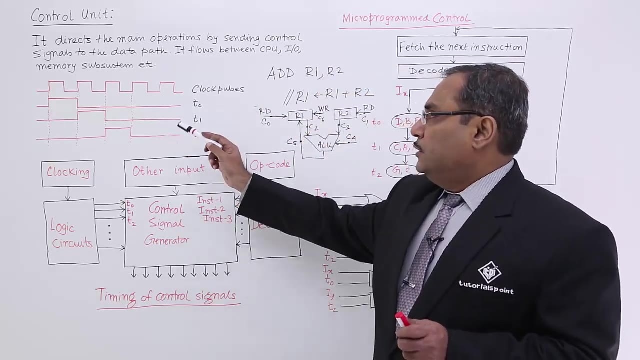 just drawing the block diagram. so that will be a black box to us. We cannot see what is actually deciding. what is the complicated circuit residing in that control unit? We are taking this one as a black box or block diagram, But the circuit will be tremendously complicated. So now for the first. 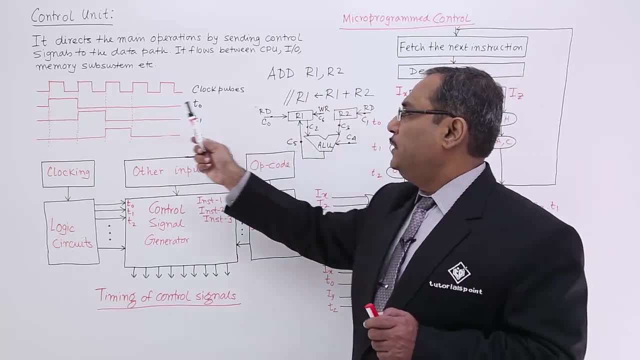 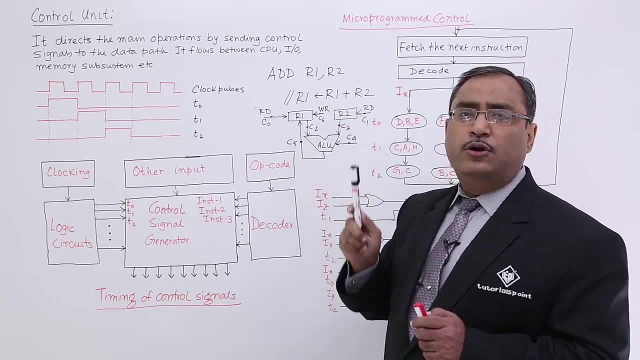 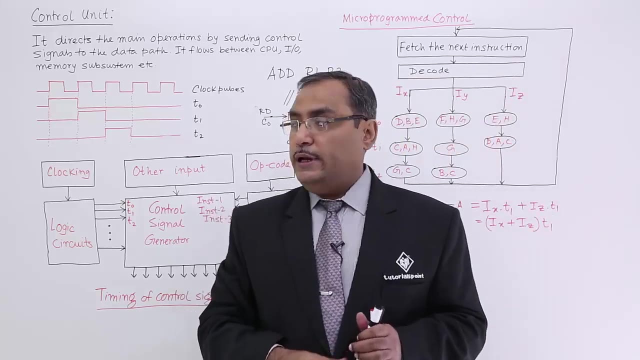 time period, the C0 and C1 should be enabled in the second time cycle. Then I should make this say this: C2 and C3 will be enabled. Then in the third cycle C4 will be enabled. so this listing will be done accordingly. So it has. 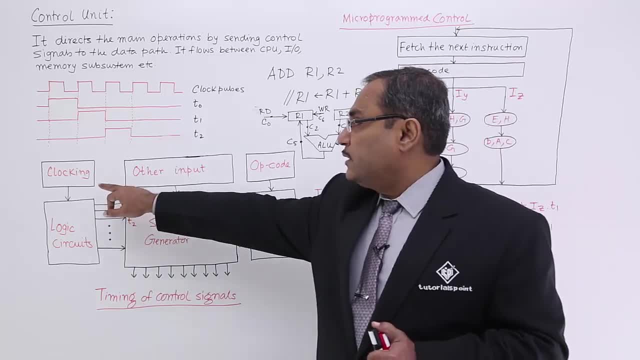 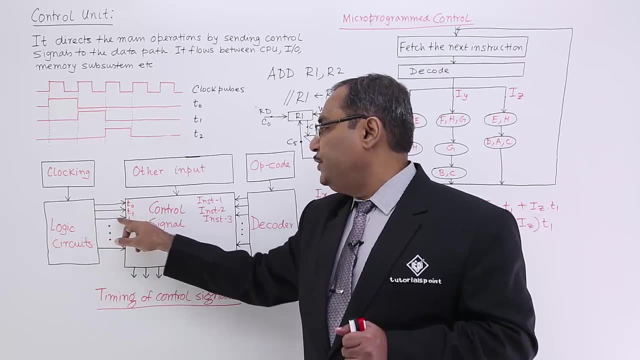 been depicted in this particular diagram, So this is a clocking From there. I will be having this: say T0, T1, say T2 and dot, dot, dot, dot. in this way, You know the meaning of this: T0, T1, T2. I have discussed. 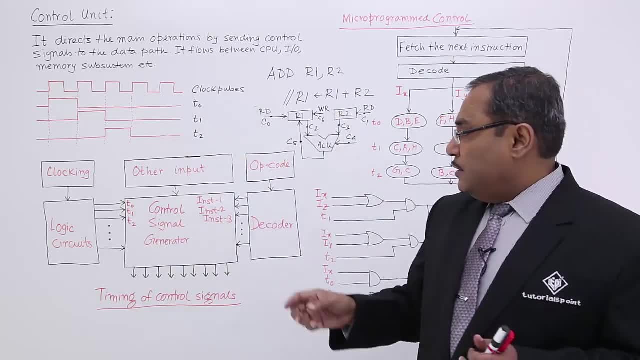 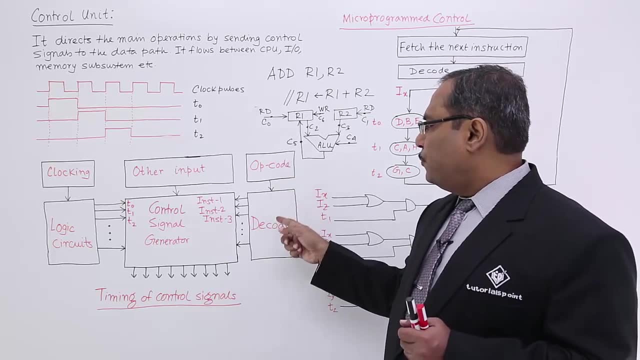 This is the control signal generator circuit. So now opcode is being kept in this particular register. operation code means instruction, So this opcode will be decoded because until and unless we decode the opcode, we cannot get the meaning. what is the purpose of the opcode? And after getting decoded? 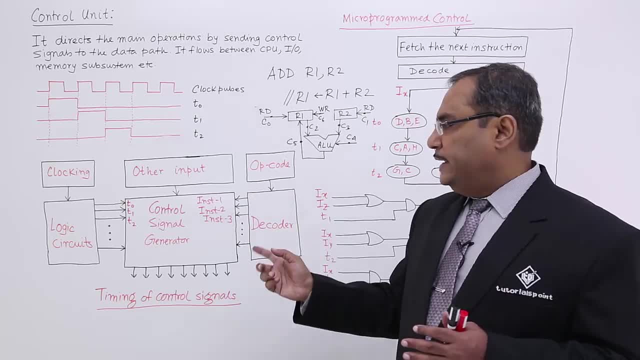 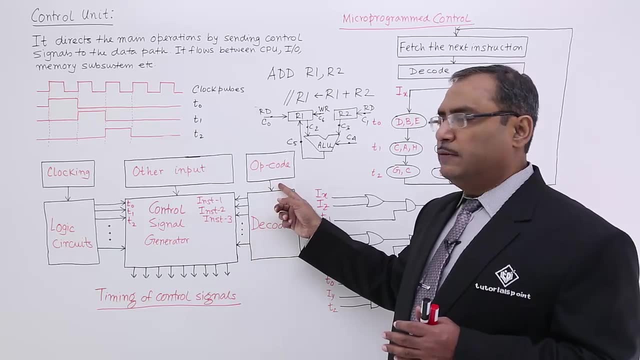 one of the output lines of this decoder will get enabled. Decoder is a combinational circuit which will have n number of input lines and 2 to the power of n number of output lines. Depending upon the voltage combination at the input, one of the output lines will be selected. That we read in: 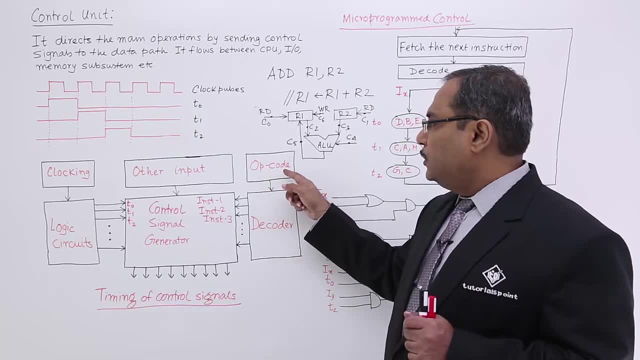 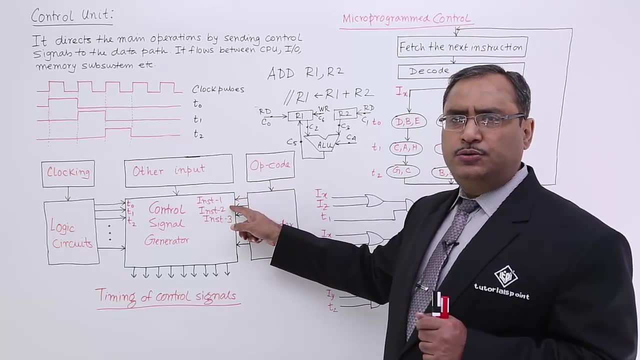 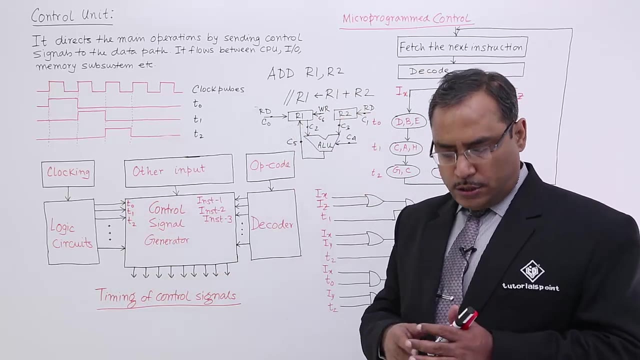 our digital electronics classes. So, depending upon the opcode, any one of the outputs will get selected by the decoder. So let it be instruction 1, or say instruction 2, or say instruction 3, and so on. Depending upon that, the control signals will get generated. So what are they? They are: 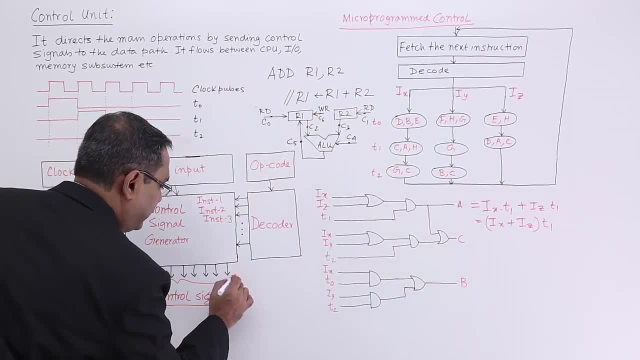 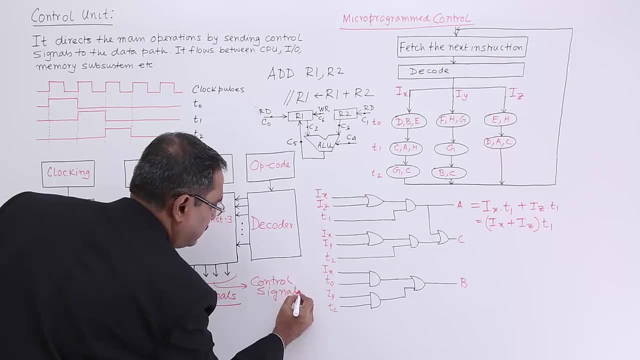 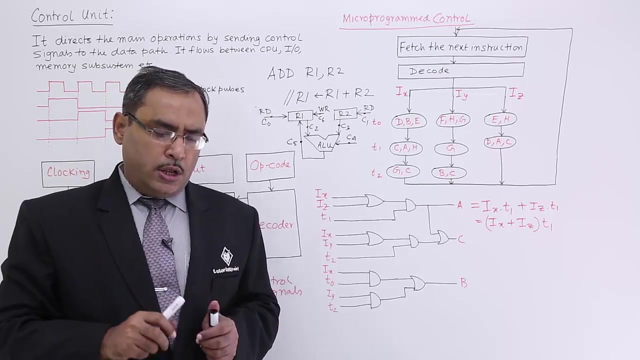 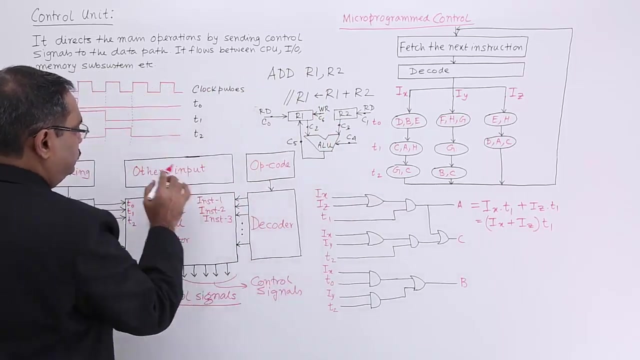 nothing but the control signals. What are they? You can also write in this way: They are nothing but the control signals. So I think you have got the logic here How this control signals are getting generated. Control circuits can be fabricated in 2 different ways. One is a micro programmed control. So I am writing: 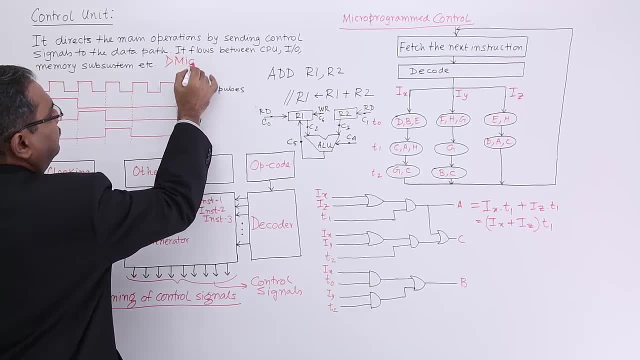 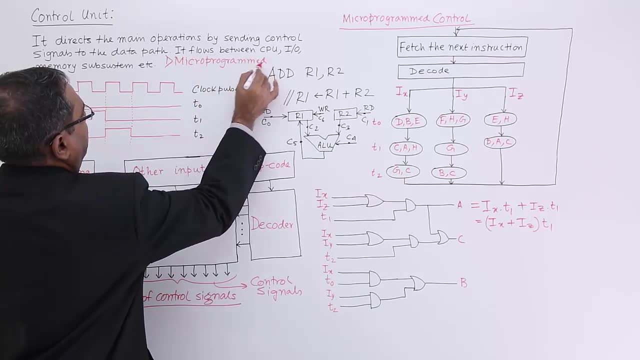 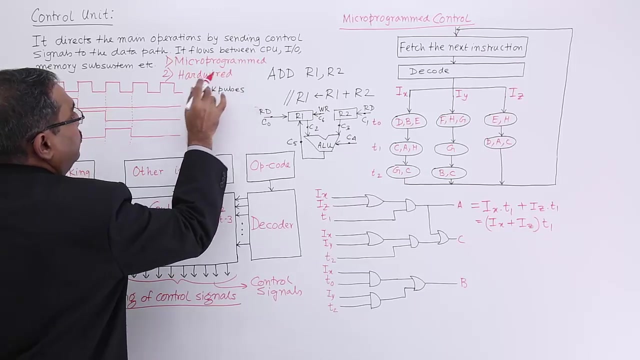 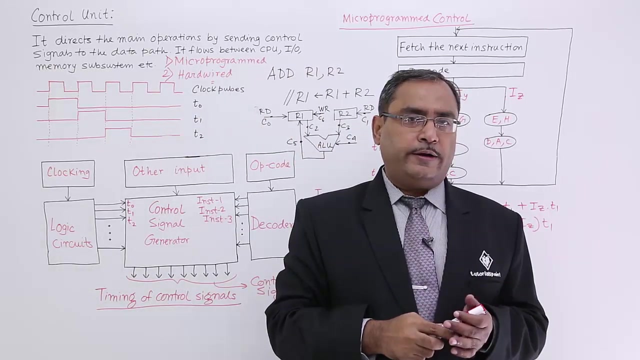 this one here say: One is a micro programmed and another one is a hardware controlled. Look at the spelling of hardware please. So this is a hardware control. So 2 types of control circuits are to be fabricated. So in our next video we shall go for this micro programmed. 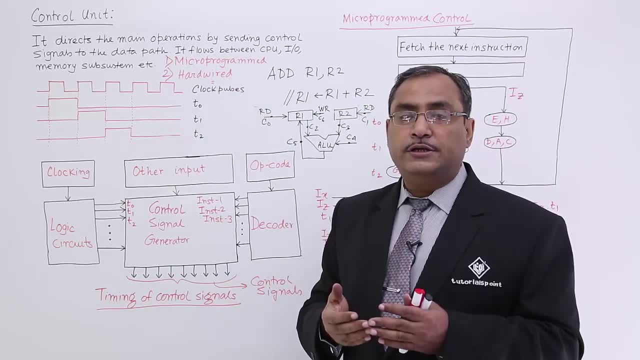 control, So how the micro programmed control circuit can generate it. Then I shall go for the hardware control circuit as well. Please watch my next videos. Thanks for watching.